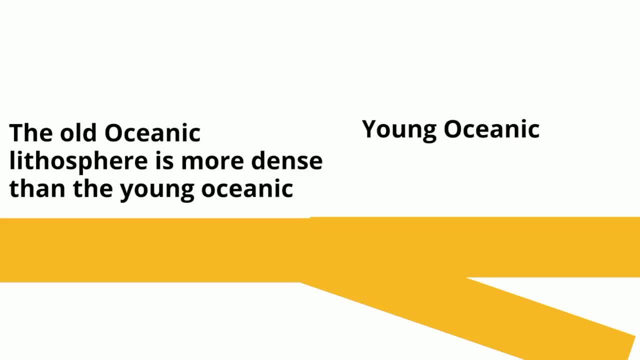 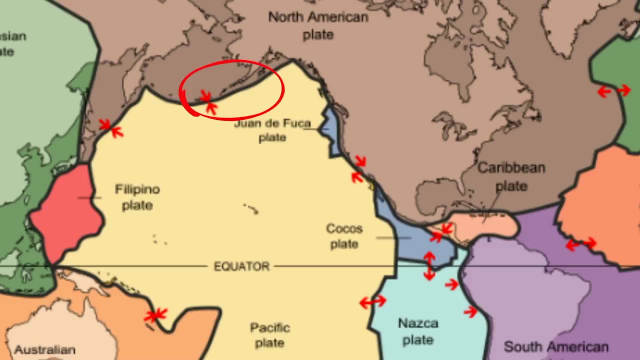 The oceanic crust is more dense than the younger crust and subducts underneath. As it subducts, magma begins to rise to the surface and this can create volcanic island arcs. An example is the portion of the North American plate covered with ocean subducts underneath the Pacific Oceanic Plate. 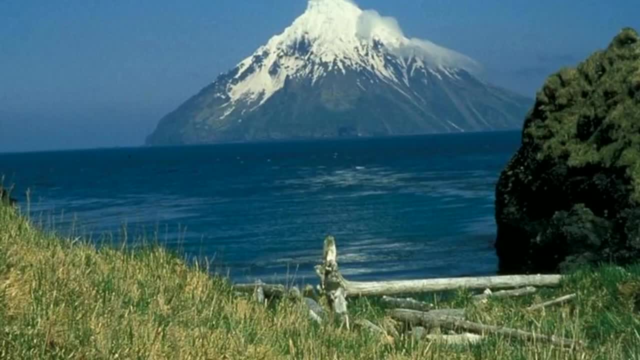 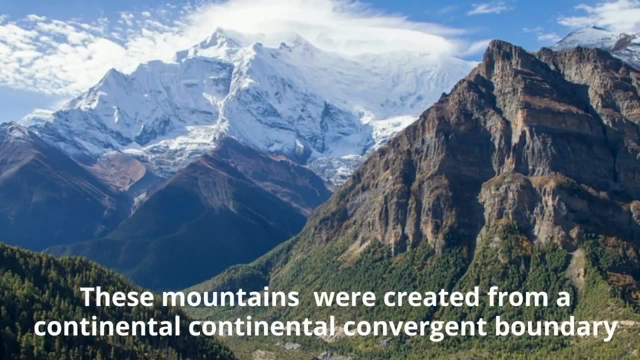 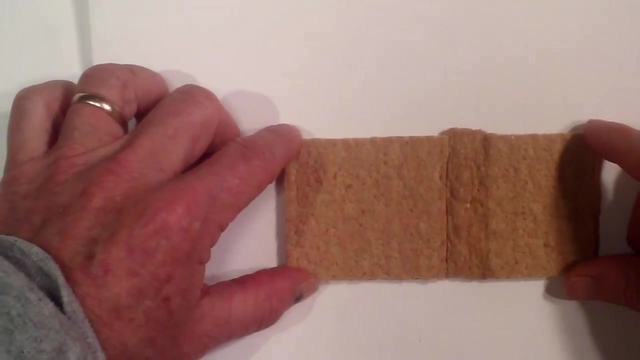 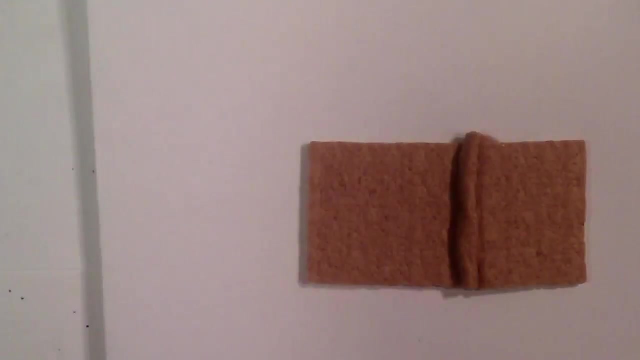 The Aleutian Islands have been created from this collision. When continental strikes, continental lithosphere, neither crust subducts Nor is magma or earthquakes occur. These two graham crackers illustrate what happens: The two plates buckle and create folded mountains. 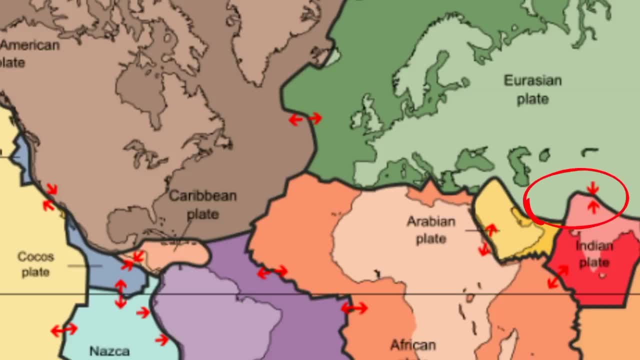 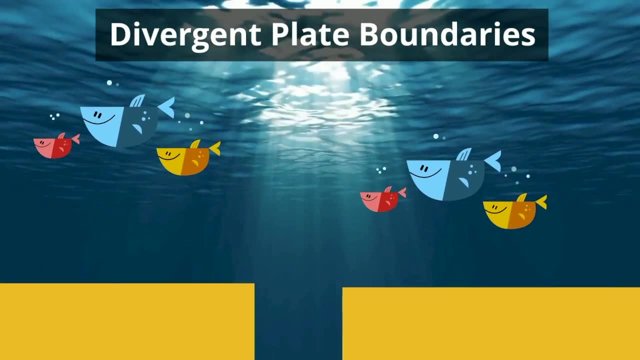 An example is the Indian plate colliding with the Eurasian plate and creating the Himalayan mountain range. Divergent plate boundaries occur where huge tectonic plates move away from one another. Divergent plate boundaries occur where huge tectonic plates move away from one another. 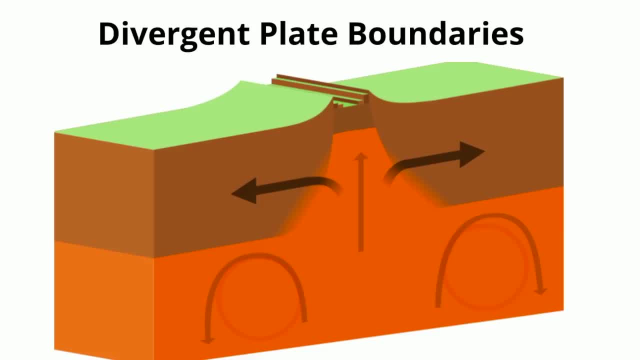 This occurs above rising convection currents. The rising magma pushes up on the bottom of the lithosphere and flows laterally beneath it. This lateral flow causes the plates to move in the direction of the flow. At the plate boundary, the two plates move in opposite directions. 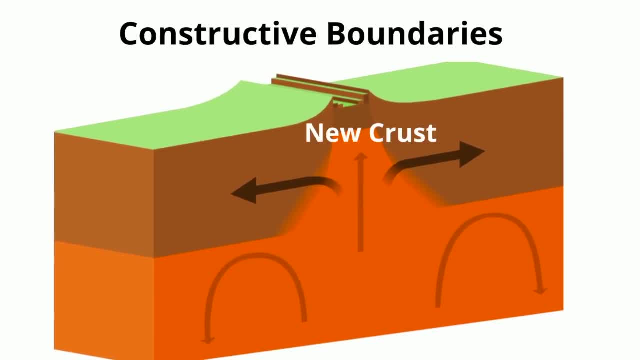 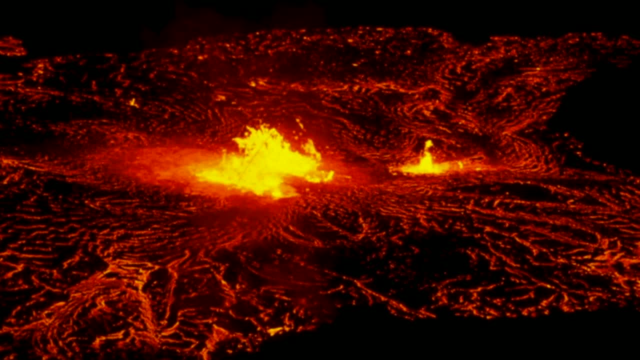 Divergent boundaries are constructive boundaries because new crust is formed As the plates move apart. molten magma fills in the gap and creates new crust. If you look at the map of the major tectonic plates, you will see that the plates move in opposite directions. 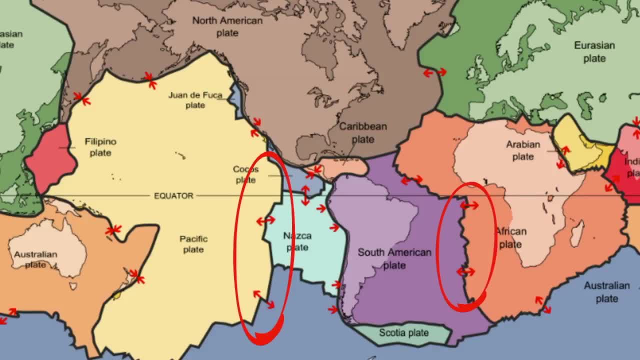 The plates move in opposite directions. If you look at the map of the major tectonic plates, you will see that the plates move in opposite directions. If you look at the map of the major tectonic plates, you will see that the plates move in opposite directions. 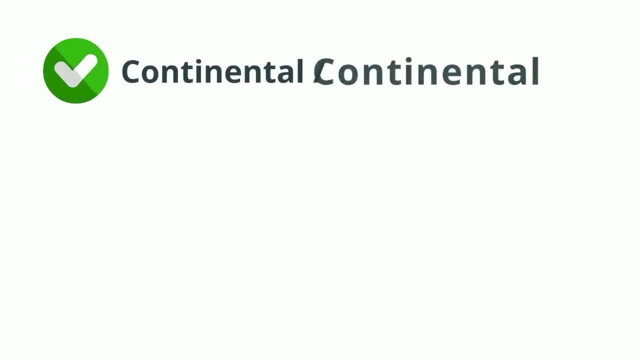 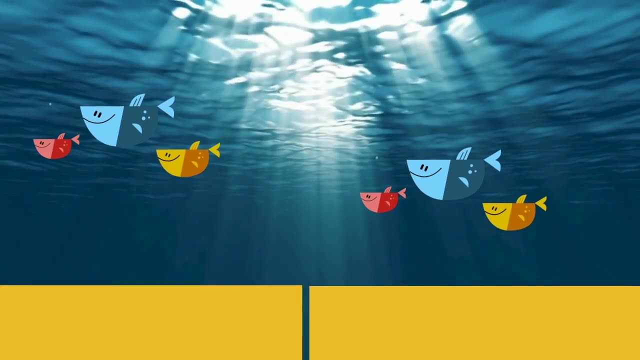 There are two major types of mandated plate boundaries: Continental and continental lithosphere And Oceanic and Oceanic lithosphere. The Oceanic and Oceanic都是 crunchy: Oceanic and Oceanic. Bisdir Francisco occurs where two oceanic plate moves away. 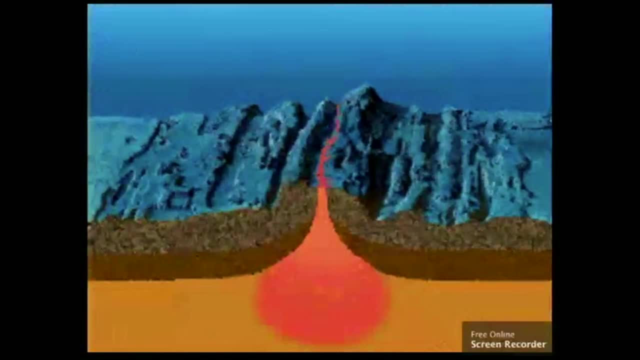 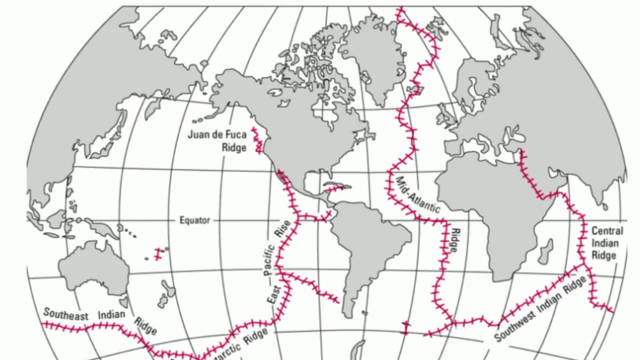 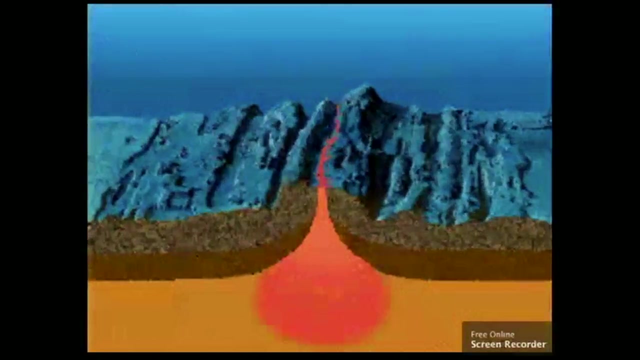 Two Oceanic plates move away from one another. This sees where seafloor spreading will occur, ridge which stretches around the world- The mid-ocean ridge- can be seen here in red. Divergent boundaries are constructive boundaries because the rising magma creates new oceanic.